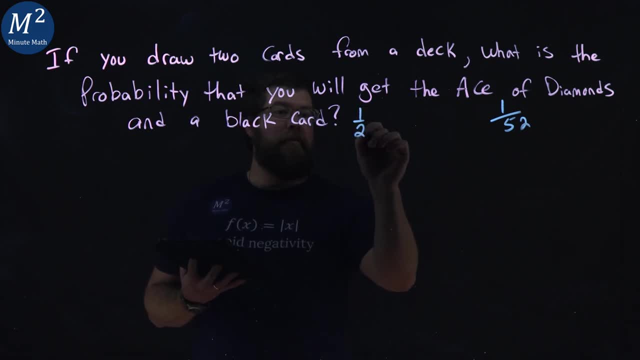 the deck. Well, that's half of them. One half or, if you want to see it as a fraction out of the 52, there's 26 of them. There's 26 black cards out of 52 in the deck. Now, this one's a little tricky. 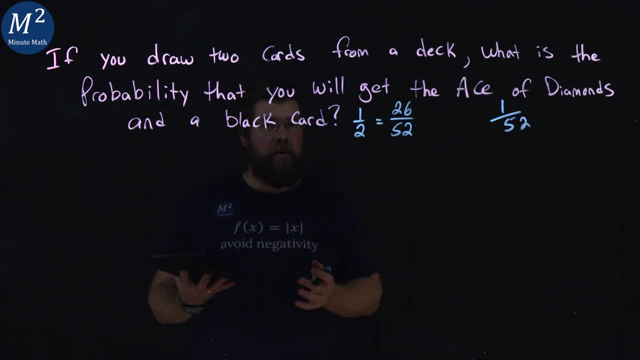 because order kind of matters. We have two different scenarios. We have one scenario where we draw the ace of diamonds first, then the black card, and flip that black card first, then the ace of diamonds. So let's go find each one of these. 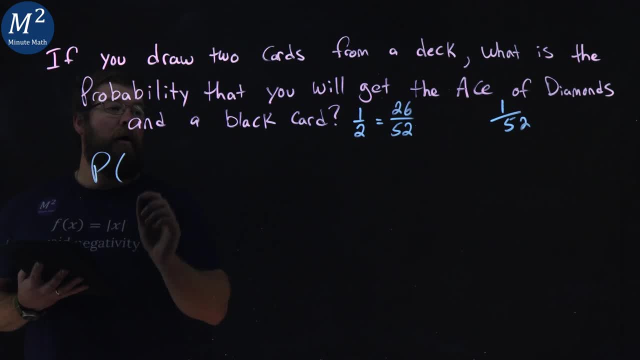 One of those out. Our first one, Our probability: this is our case A, our first case here. Our probability: we have the let's go- ace of diamonds and black. So that's our order. Ace of diamonds first has a probability of 1 out of 52.. We multiply that by 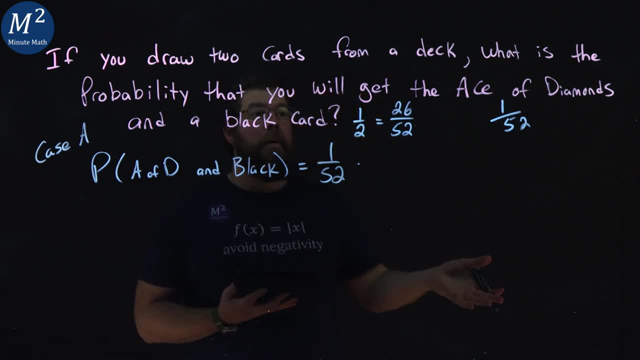 the probability of getting a black card. Well, one card is already out of the deck. Ace of diamonds is out of black cards, so we don't have to worry about that. changing just the total number of cards in the deck: 52 becomes a 51, and there's still 26 black cards left over. This multiplies. 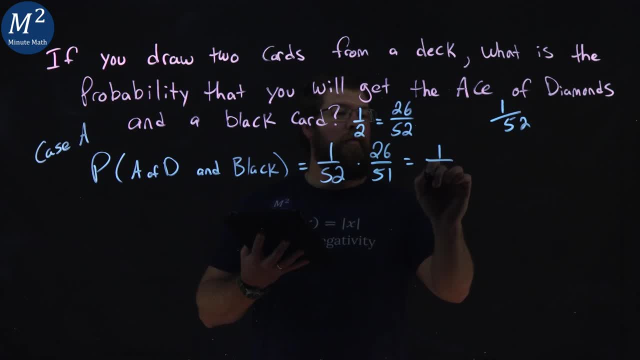 out to be a simplified a 1 over 102.. Now our second case is the other probability here: Black card first and then our ace of diamonds. So we have a black card first and then our ace of diamonds. Well, the probability of a black card first: 26 out of 52. Multiplied by now, there's only one ace of diamonds and there is now one card out, one black card out. so there's 51 cards left in the deck. Now, if you look here, this is the same multiplication problem that's happening. This is also a 1 out of 102 chance.